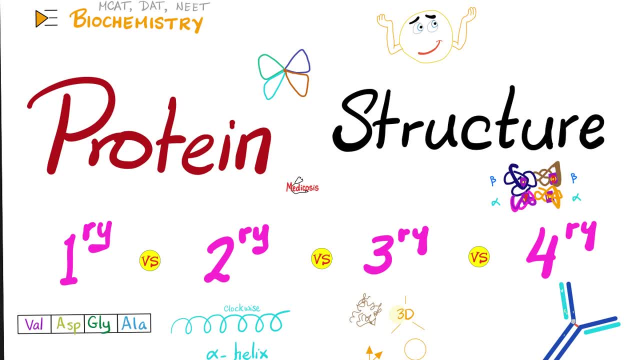 to talk about the protein structure from simple to complex. let's go primary, secondary, tertiary and then quaternary structure. the primary protein structure is just a sequence of amino acids. how about the secondary structure? this is number two, because secondary has two types: the alpha helix. 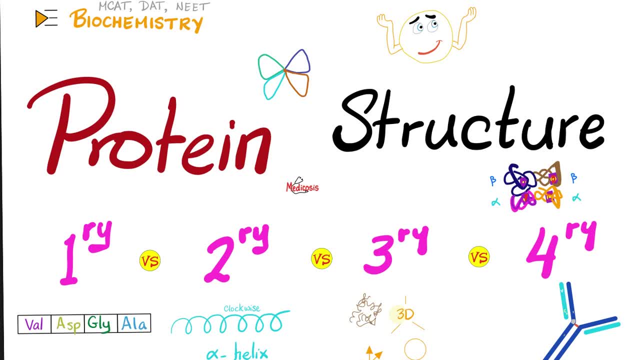 and the beta pleated sheets. next is the tertiary, which is the three-dimensional shape of the protein. and last is the quaternary structure. by the way, not every protein has this. you gotta have at least two or more peptide chains to have it. example is the reduction of amino acids. so you can keep theQUATERNARY structure in there. 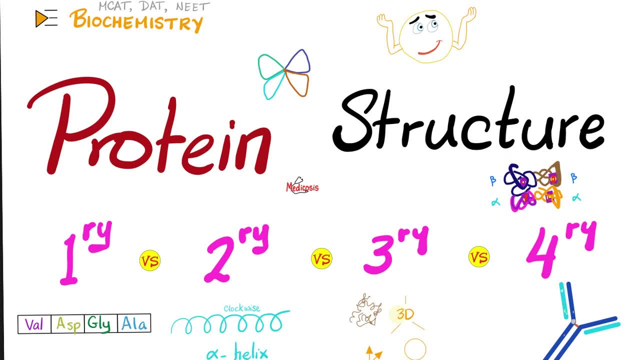 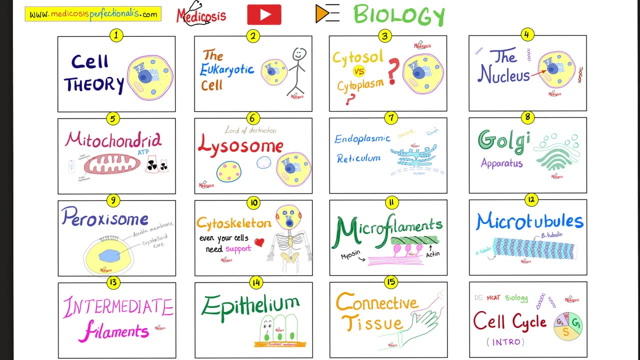 the hemoglobin because it has two alpha subunits and two beta subunits. that's a quaternary structure. also, antibodies: they have two light chains and two heavy chains- a quaternary structure. this is my biochemistry playlist. please watch these videos in order and please watch this playlist after. 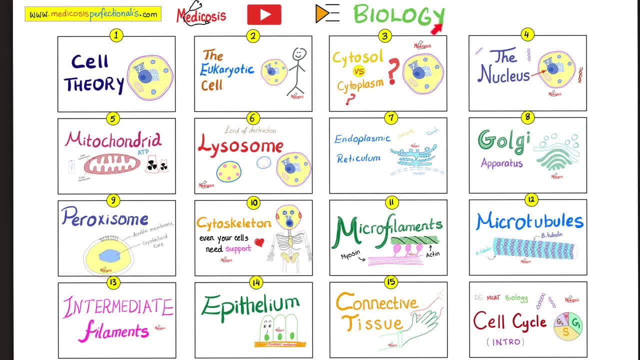 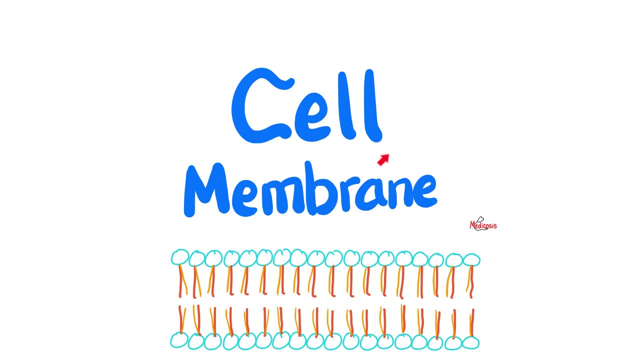 finishing the biology playlist first. biology is so easy, much easier than chemistry or biochemistry. so if i were you, i'll start with biology as early as possible so that i can focus on chemistry next, while doing biology question in review and because we will use lots of biology info to understand. 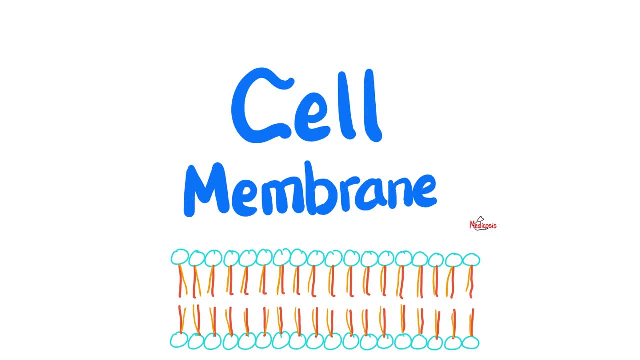 biochemistry. you don't believe me. consider this: the cell membrane. remember the hydrophilic head, hydrophobic tail. and why is that? because there is water on the outside and water on the inside of the cell. so i'll put the hydrophilic towards the water. 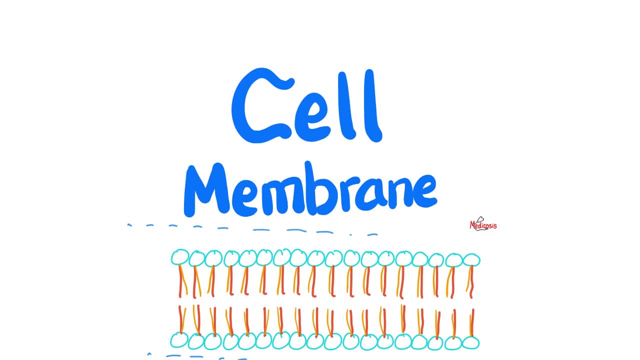 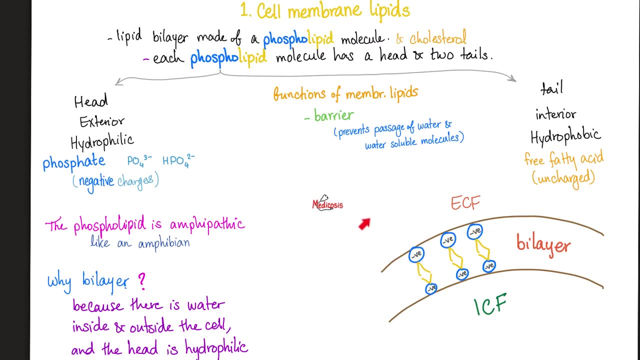 on the outside and on the inside. how about the lipid? who hates water? i will bury the fat in the middle, and that's why you need a bilayer, because there is water outside and there is water inside, and the fat is always buried in the center. that's why your cell membrane is like an amphibian. 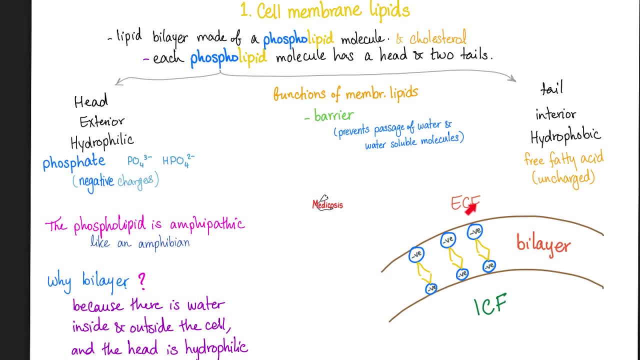 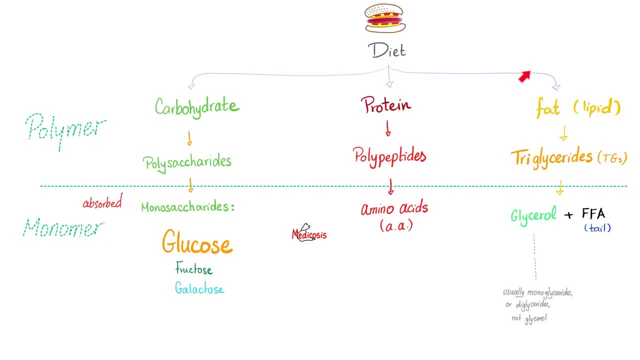 it's amphipathic. five minutes from now, we will use the same concept in the tertiary structure of protein. next, recall that your diet is carbs, proteins and fats. proteins become polypeptides, and then oligopeptides, dipeptides and then amino acids, which is just a monopeptide. how about fat or lipid? they start with triglycerides. that's the big fat. 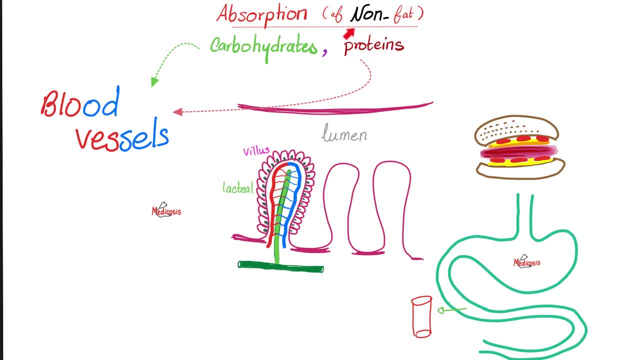 then they become glycerol and free fatty acids. how to absorb anything that is not fat, ie not lipid soluble, ie water soluble, easy into blood vessels, arteries and veins. but what if i want to absorb fat? oh oh, that's a different story. i'm going to show you how to absorb fat and how to. 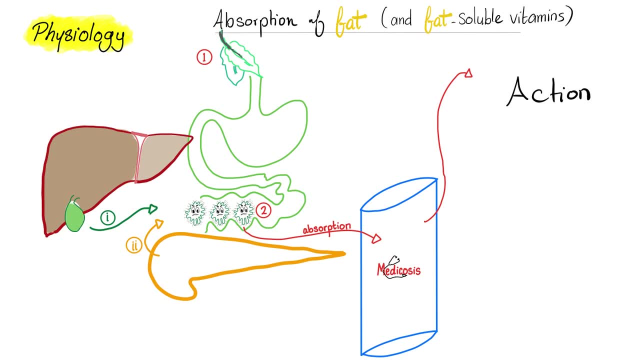 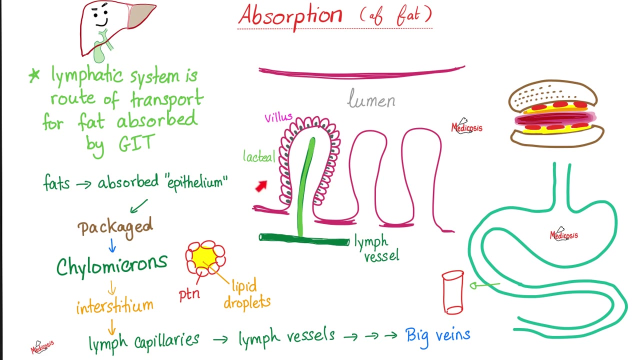 absorb fat. to absorb fat, you need three organs to be robust. one, liver and biliary system, two, pancreas. three, the bowel or the intestine, which will do the actual absorption. when you absorb fat, you do not go into blood vessels. instead, you go into lymph vessels, such as these wonderful lacteals. 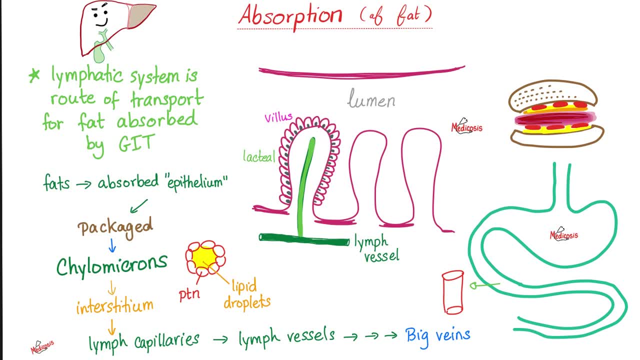 in the villi of your intestine and look at this. you bury your fat in the middle and you put the water soluble stuff on top of it and you absorb fat. you do not go into blood vessels. instead, you put the water soluble stuff on top of it and you put the water soluble stuff on top of it and you. 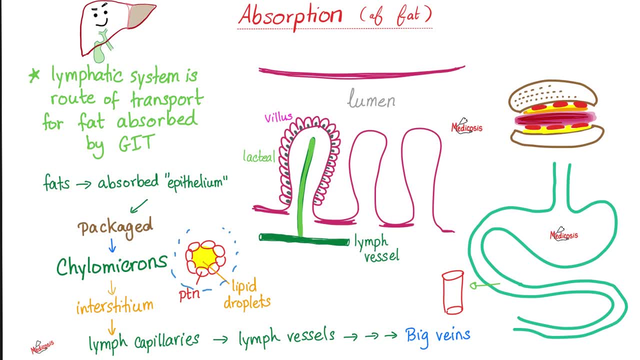 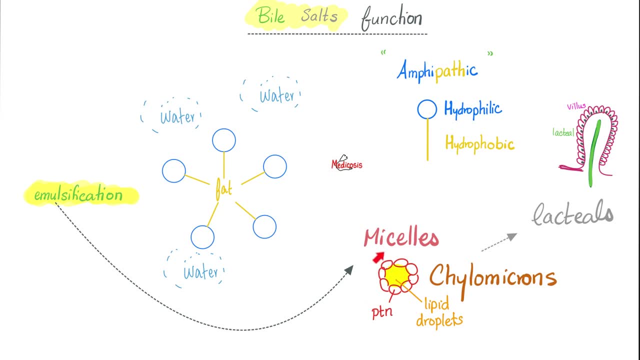 the outside. you know why? because there is water on the outside everywhere. what's the name of the wonderful structure that made this organization? thank you, bile salts, for making those micelles. then you package me into chylomicrons, send me to the lacteal, which will send me to the lymphatic. 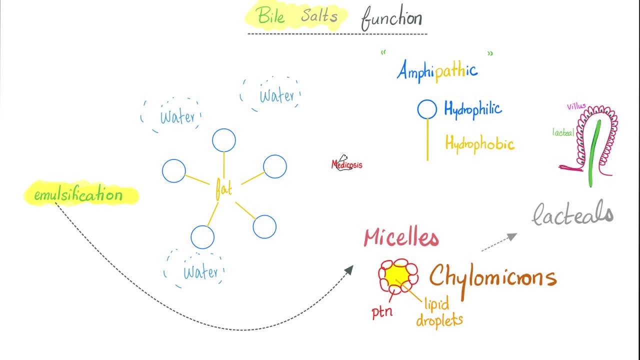 vessels which will eventually send me to thoracic duct on the left or right, lymphatic duct on the right side. eventually, both will end up into big veins which will take us to the right side and the right atrium of the heart. this concept of hiding the fat on the inside while leaving the 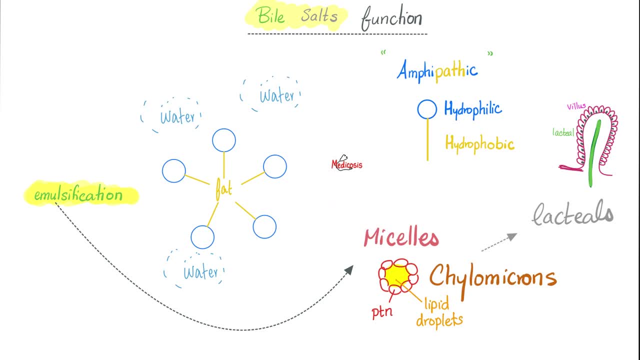 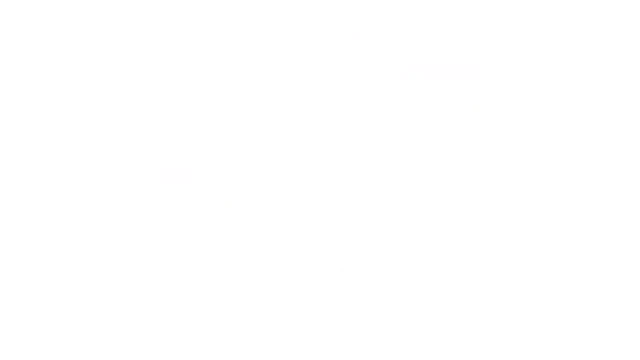 water soluble on the outside is going to be used again five minutes from now when we talk about the tertiary structure of proteins. now please get your gluteus maximus off the couch and draw this with me using pen and paper. let's draw the structure of the amino acid. you start with a carbon- amazing. 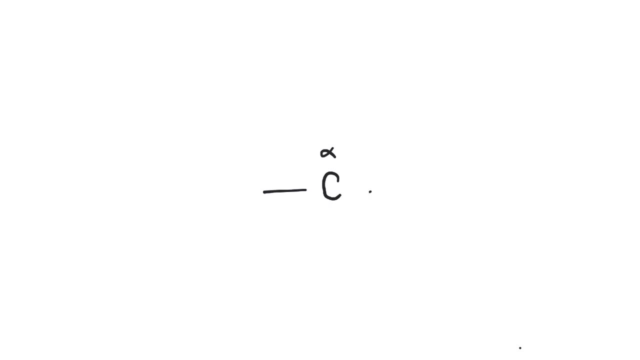 this is called the alpha carbon. and then left versus right. remind me please, what are we trying to draw? amino acids. say it again, because it was so beautiful. amino acid, correct amino acids. you start with amino on the left side and you go with the acid on the right side. recall from chemistry that carbon requires four bonds. here is one. here is: 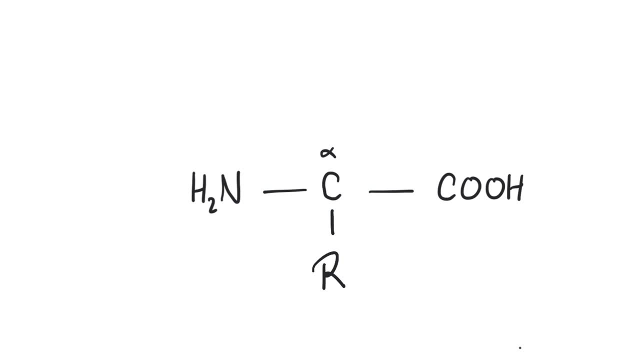 two, all right. the third one is attached to an r group, which could be anything, and the last one is simply hydrogen. this is the structure of your amino acid. easy peasy. pause and review. since we say amino before the acid, since a comes before c, you start with the amino and then the acid. this order matters. who determines the chemical properties of? 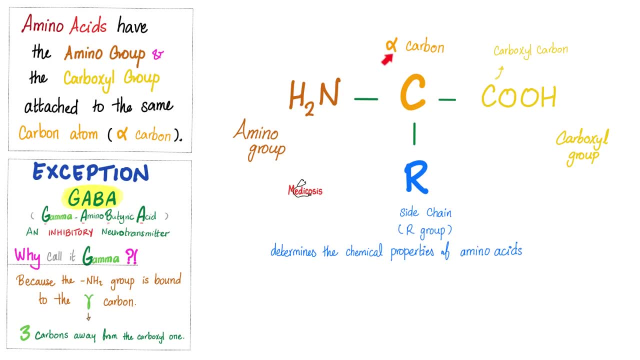 the amino acid, the r group, the side chain. this is the alpha carbon, unless you're gaba, where your amino group is bound to that gamma carbon. that's why we called gaba, because it stands for gamma amino butyric acid, as we have discussed in the previous video. so let's start with the alpha carbon. 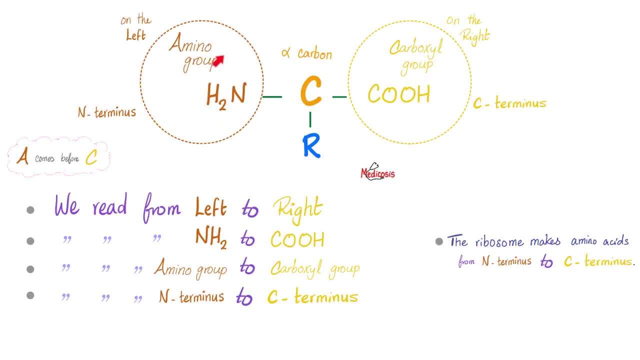 in this biochemistry playlist and when i say that you start with the amino and then you follow it by the acid, this is not an arbitrary order, it's not a quote, social construct, unquote. it's actually how the ribosome makes the amino acid. the ribosome itself starts with the n-terminus and ends with. 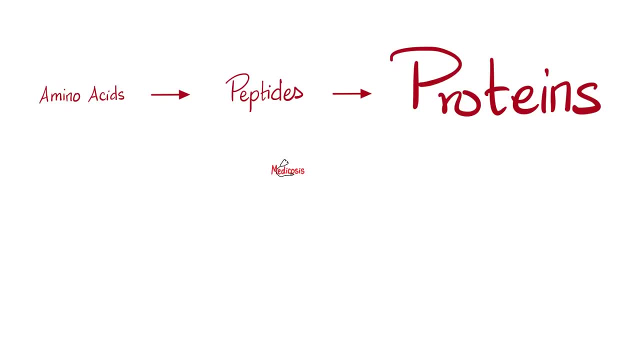 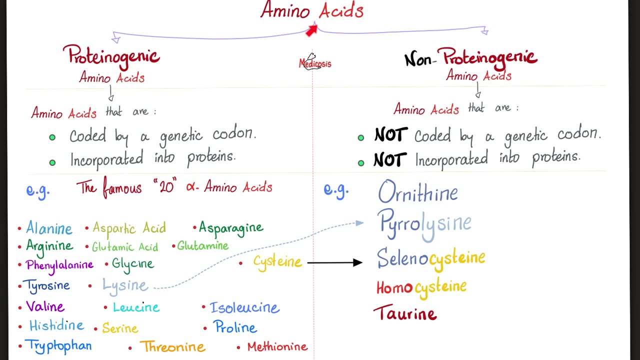 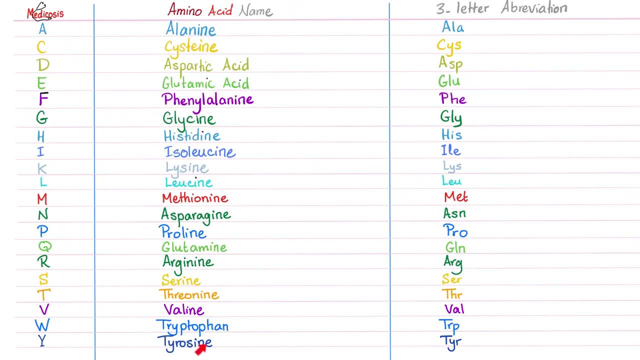 the c-terminus. if i lump a group of amino acids together, congratulations, you have peptides. lump those peptides together, you get proteins. are all of the amino acids in the body incorporated into proteins. no, only the 20 proteogenic famous amino acids are the ones incorporated into proteins and the ones coded by your dna. each one has a name, a one letter. 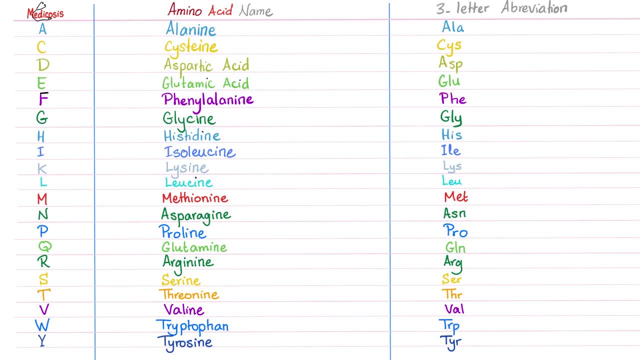 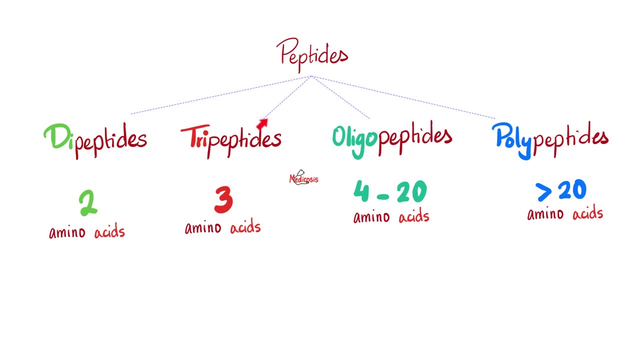 abbreviation and a three letter. abbreviation, pause and review. and again, what kind of peptides are you talking about? could be dipeptides if you're made of two amino acids, tripeptides, three amino acids, oligopeptides, four to twenty, polypeptides more than 20.. but what's the mono peptide then? that's just one amino acid, doofus, pause. and 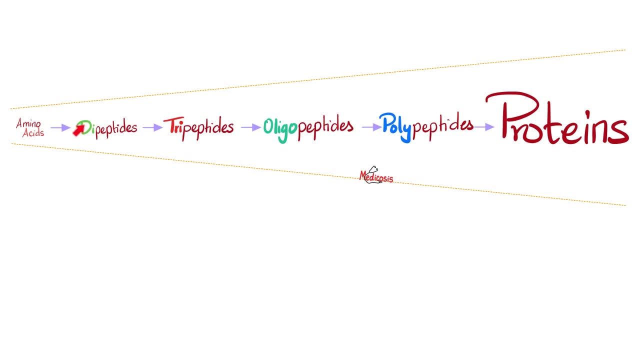 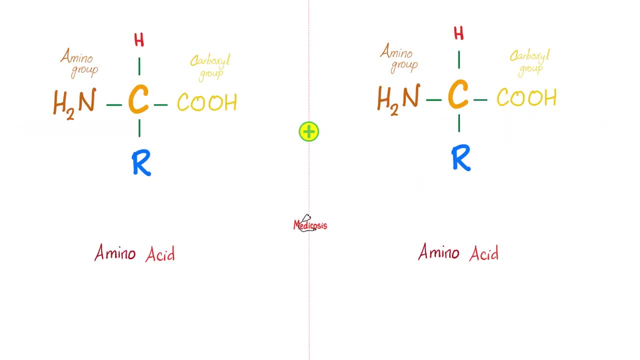 review. so there you go, here's your amino acid, and then lump two together: dipeptides, and then tripeptides, oligopeptides, polypeptides and then proteins. but how do you lump them together? by forming a peptide bond. you see the carboxyl group of this amino acid and the amino group of the next. 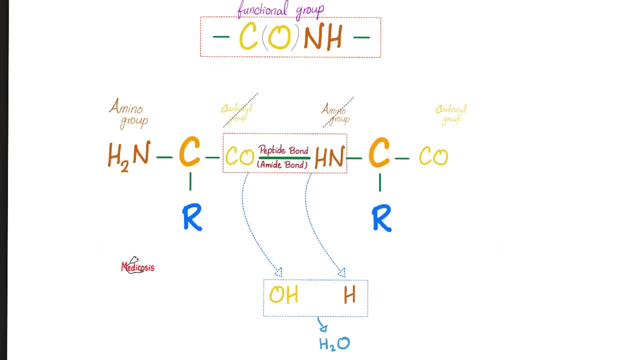 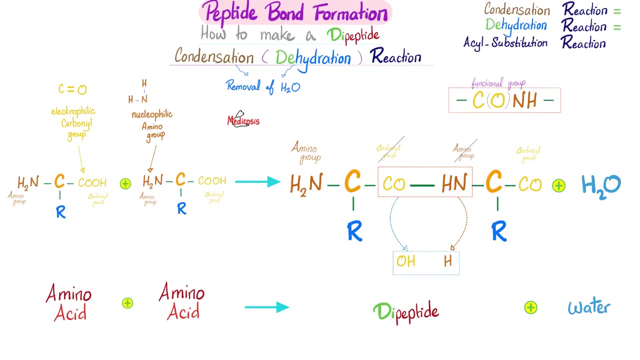 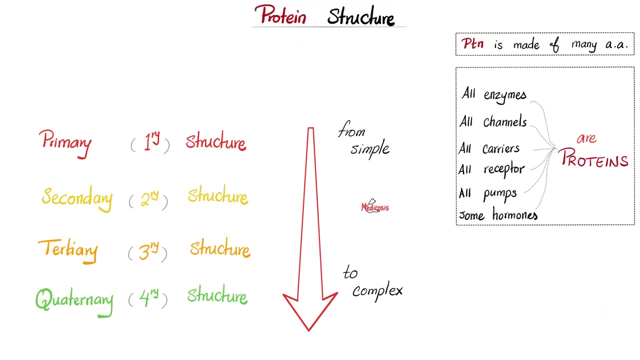 amino acid. let's remove the oh from the first and the h from the second to make water, and what's left is going to make a peptide bond, also known as amide bond, giving you this functional group right here. because this reaction yielded water, you can call this a dehydration reaction. now you're ready to understand the protein structure. proteins are. 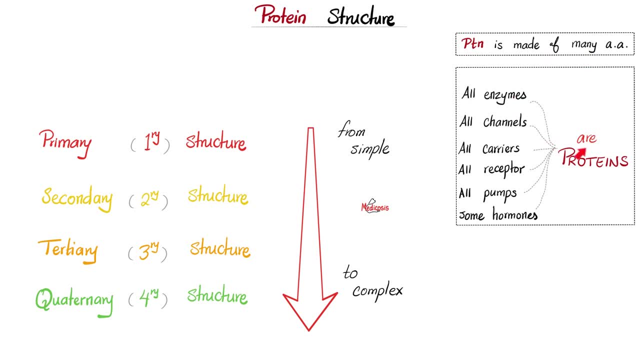 made of many amino acids. as you know, all enzymes of your body are proteins, all channels proteins, all carriers are proteins, all receptors are proteins, all pumps are proteins. some hormones are proteins, the others are fat. but hey, medicosis, i know like about an rna inside the cell that acts as an enzyme, but it's not a protein. i know doofus. there are exceptions. 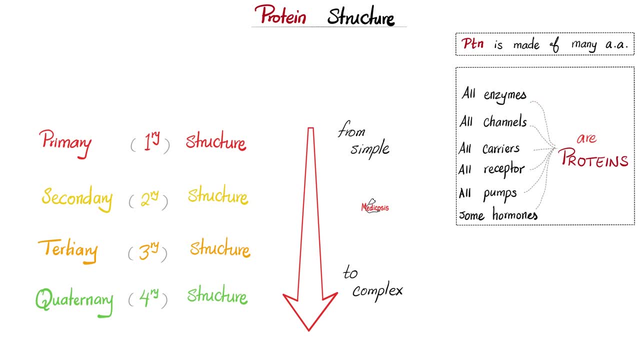 we're trying to keep it simple over here. if you want to confuse yourself, go listen to your professor. enough with these dead jokes. protein structure from the simple to the more complex: primary, secondary, tertiary, quaternary. they are color coded in my life and you can always download. 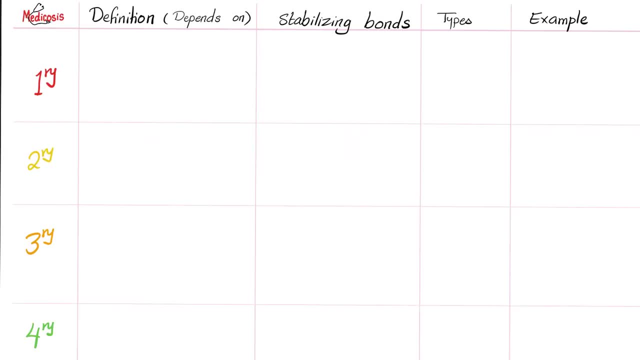 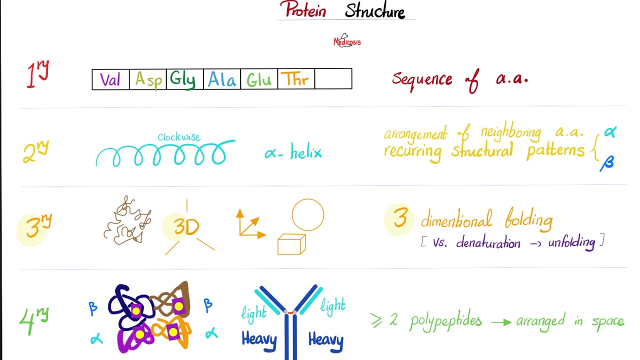 these notes at medicosisperfectionistcom. by the end of the video, you should be able to fill in this table. i'll show you how to do it at the end, but just watch the video and try to fill in the gaps. it will be better for you if you can do it yourself. primary protein structure. what the flip is that. 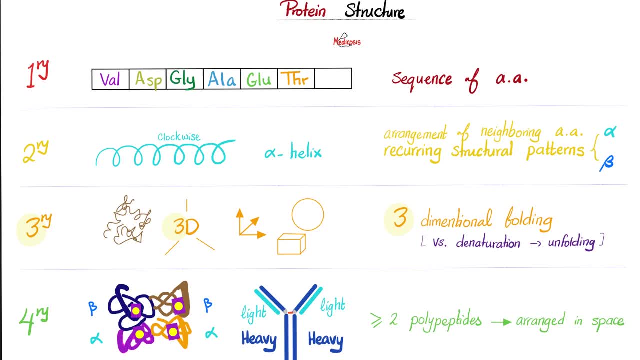 it's just the sequence of amino acids, that's it. yeah, hey, medicosis, does it matter that aspartate comes after valine, not valine after aspartate? yes, of course it matters. it's about the sequence of amino acids, that's it. yeah, hey, medicosis, does it matter that aspartate? 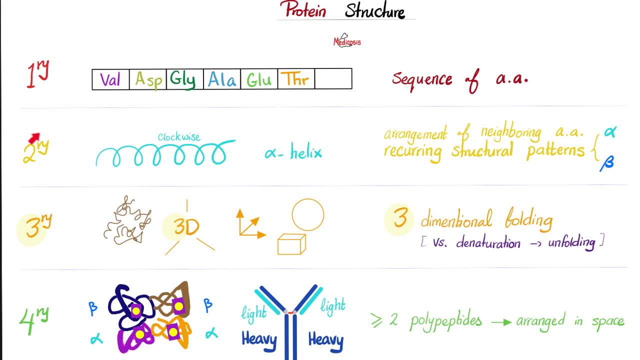 comes after valine, not valine after aspartate. yes, of course it matters that aspartate sequence dude. this is important. how about the secondary protein structure? just remember number two, because we have two patterns here: the alpha helix and the beta pleated sheets, which are 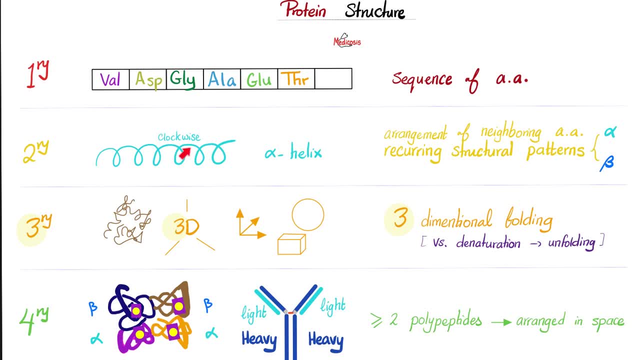 nothing more but arrangement with the neighboring amino acids. to give you these recurrent structural patterns. hint, the alpha helix rotates clockwise. third, tertiary protein structure. just remember number three for 3d, three-dimensional folding. and please try to keep this in mind because in a later video we'll talk about protein denaturation, and i will remind you that protein denaturation is. 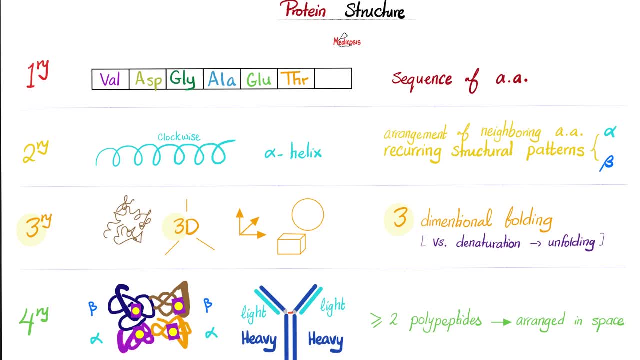 the exact opposite of the tertiary structure. in tertiary structure we're trying to fold the protein, but in denaturation we're trying to unfold it. integration, disintegration, the one in the many versus the many without the many, and the one in the many without the many and the one in the many. without the one that was deep last. quaternary structure: not every protein has a quaternary structure. if you want a quaternary structure, you've got to have at least two polypeptides. you could have two or more. you can have a hundred if you want, and these are arranged in space. 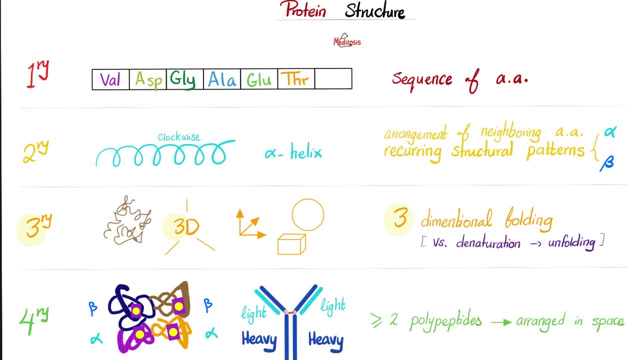 example, hemoglobin: two alpha chains and two beta chains. mnemonic, two plus two equals four. how about this? this is the antibody, also known as aminoglobin, which is a gamma globulin, if you remember your biology. this aminoglobin has two light chains and two heavy. 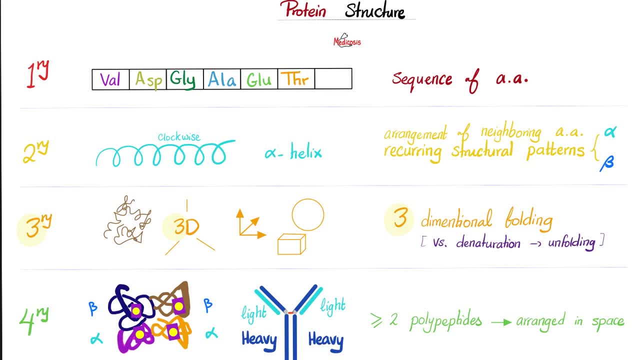 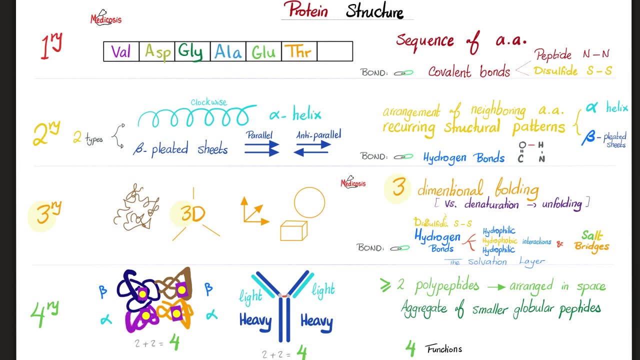 chains. mnemonic two plus two equals four. quaternary structure: let's take it to the next level: primary protein structure. what's that sequence of amino acid? what's the name of the bond that's keeping them in place? covalent bonds, mostly peptide bonds, but could be disulfide as well: sulfur and sulfur. 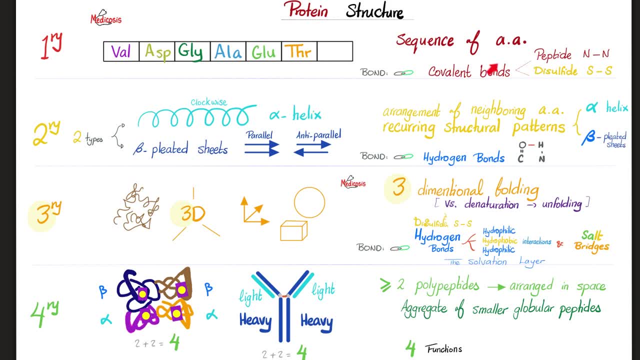 on your exam day. peptide bonds are the ones that are keeping them in place, and the ones that are keeping them in place are the ones that are keeping them in place, which are the disulfide bonds. the disulfide bonds are more important for the primary structure, while the disulfide bond are. 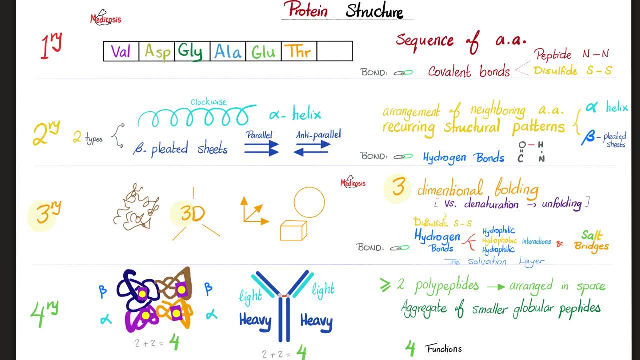 more important in the tertiary structure, next secondary, two for two, two types such as the alpha helix- remember the clockwise and the beta pleated sheets could be parallel or anti-parallel. what's keeping them in place? hydrogen bond between what? between the oxygen of the carbonyl group. 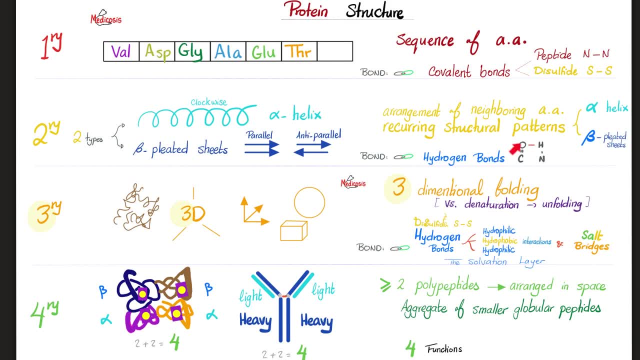 and the hydrogen of the amide group group between the oxygen and the hydrogen will have a hydrogen bond. next, tertiary structure, remember for three the 3d, and this depends on three things: hydrogen bond, disulfide bond and salt bridges, not to be confused with your three-dimensional yoga bridges. last quaternary: 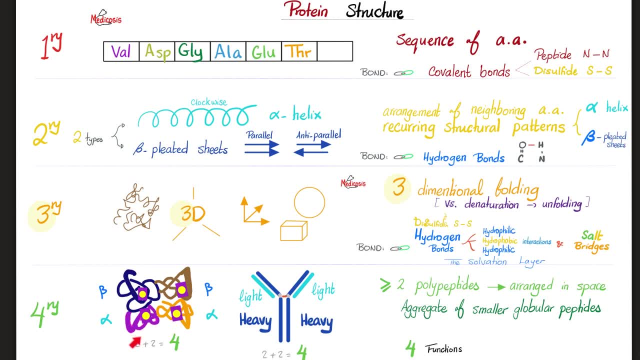 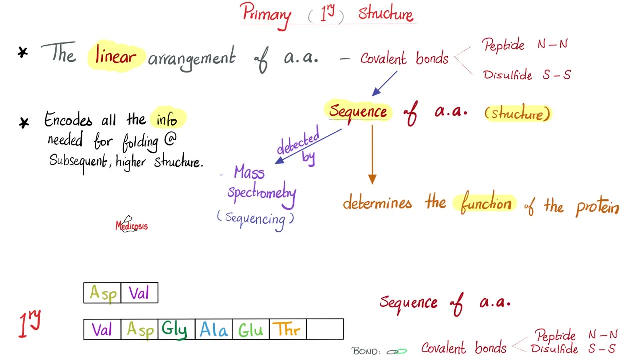 structure: two plus two is four: two alpha chains and two beta chains in hemoglobin and two light chains, two heavy chains of the immunoglobulin. the quaternary structure has- guess what- four functions, as we'll discuss soon. let's dig even deeper: primary structure: what's that linear arrangement? 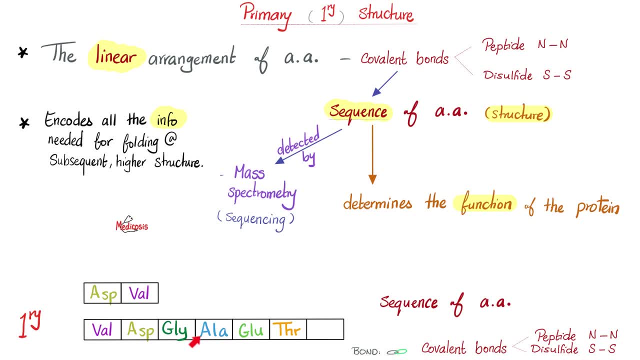 of the amino acid. the sequence matters, the order matters, since this is all the info this encodes for all the info that you need for folding at subsequent higher structures. ie you need the sequence for the next secondary, tertiary and quaternary structures that will come later. sequence of amino acid is the structure. 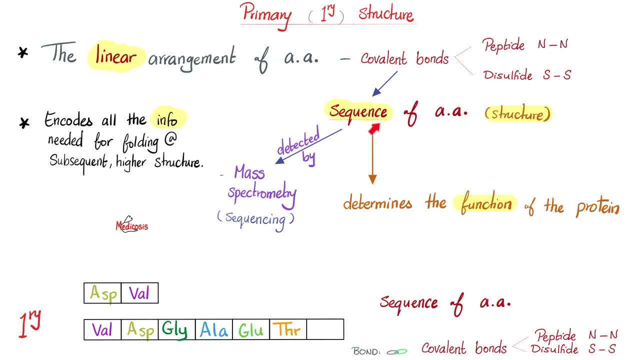 which determines the function of the protein. no kidding, how can i detect the sequence? many techniques in biochemistry- here is the crown jewel- mass spectrometry and, of course, any technique that is trying to establish the sequence will be called sequencing. what's keeping you in check? covalent bond, mostly peptide bond, between this amino acid and the following: 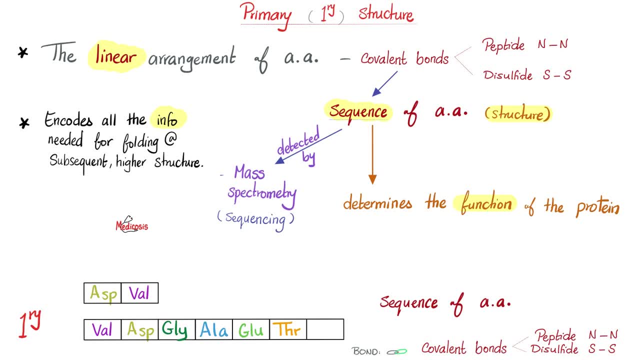 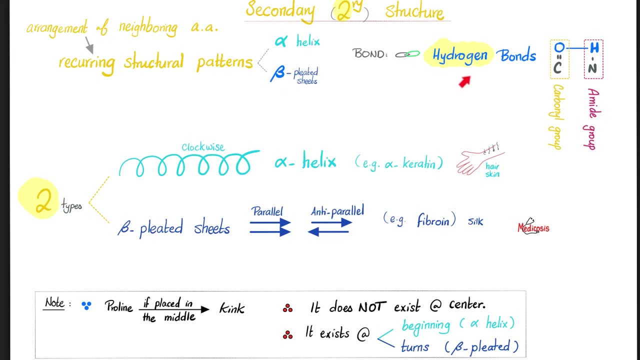 amino acid, between one amino acid and the next amino acid. number two, secondary structure which has two patterns: alpha, helix and beta pleated sheets. what's keeping you in check? hydrogen bond between two groups: carbonyl group- i need your. oxygen amide group, i need your hydrogen boom you. 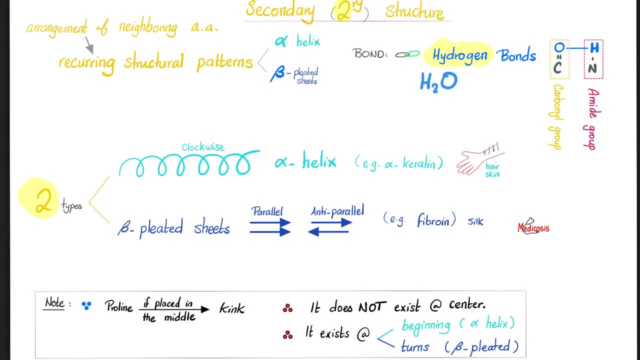 have a hydrogen bond, just like the one you have in water, guys. by the way, i think i'm being poisoned, and now i'm getting more and more out of this. you know what the name of the poison is: dihydrominoxide. please, if i pass away, call the cops because i'm in grave danger, did you believe? 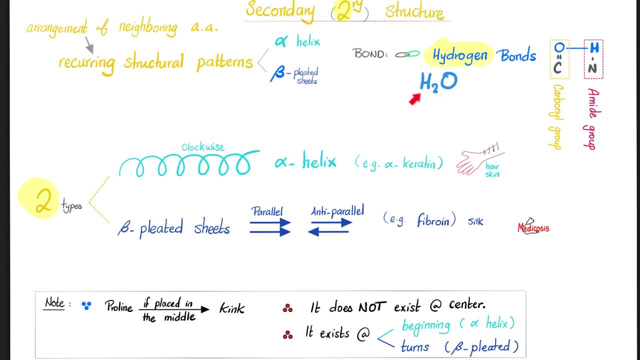 me, you freaking doofus. dihydrominoxide is just water, classic dad joke. why is anybody watching my videos? the two types of the secondary structure- remember two with two: alpha helix and beta pleated sheets. give me an example of each. alpha helix is like an alpha keratin. alpha helix is like a. 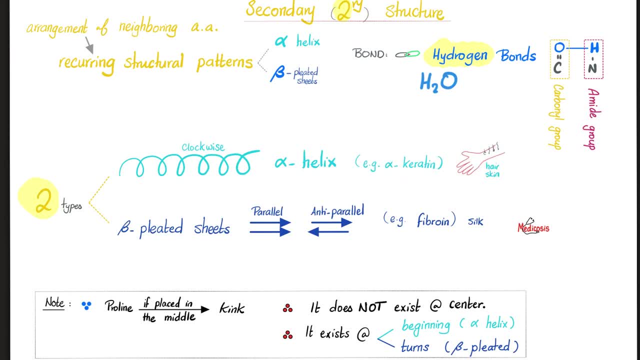 alpha keratin- alpha helix is like an alpha keratin. alpha keratin- alpha helix is like an alpha keratin which is found in your hair, skin, etc. How about the beta pleated sheets, Fibroin, which is found in silk? Why does silk have a pattern? Because it's a beta pleated sheet. Note: proline is weird. 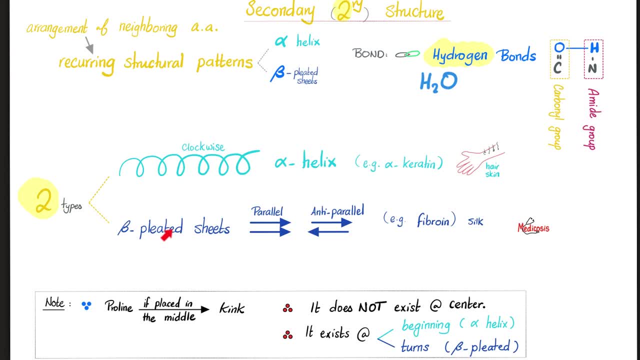 If you put proline in the middle of the alpha helix or in the middle of the beta sheet, it will make a kink and will destroy the whole thing. Therefore, proline will not exist in the center. Proline will exist at the beginning or at the start of the alpha helix or at the turn of the beta pleated sheet, but not in the middle Next to the tertiary structure. Have you ever wondered why proteins exist as fibrous proteins or globular proteins? Fibrous proteins include what? Collagen and elastin fibers? How about globular proteins? Oh, something like globulin, if you remember your. 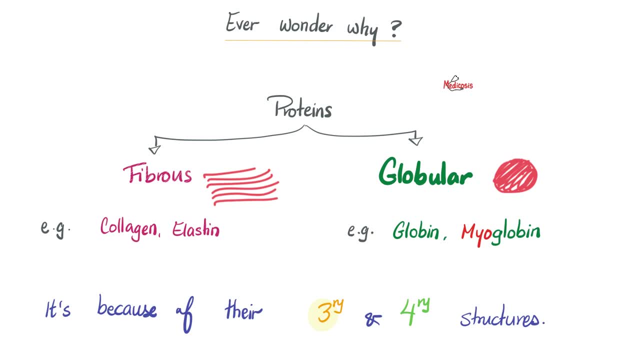 biology, or globin, also globular globin, myoglobin, etc. Do you remember albumin and globulin, the plasma proteins? Globulin is also globular. Now, do you know why proteins are either fibrous or globular? It's thanks to their tertiary and quaternary structure. Which one is. 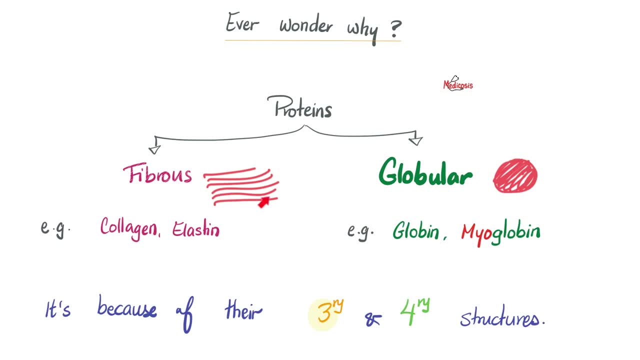 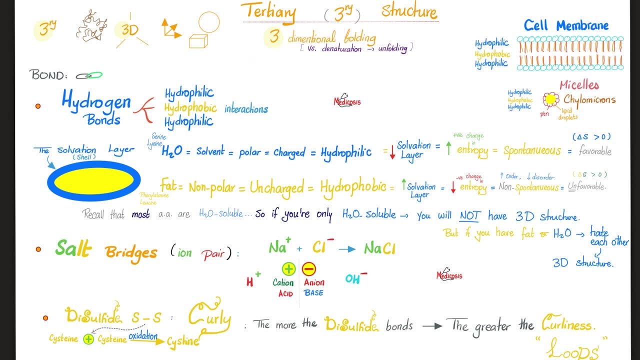 more important. Tertiary structure, because this is the three-dimensional shape of the protein. Tertiary structure, let's go Three, Three-dimensional. What keeps you in check? Three forces: Number one: hydrogen bond. Two: salt bridges. Three: disulfide bond. Let's start with. 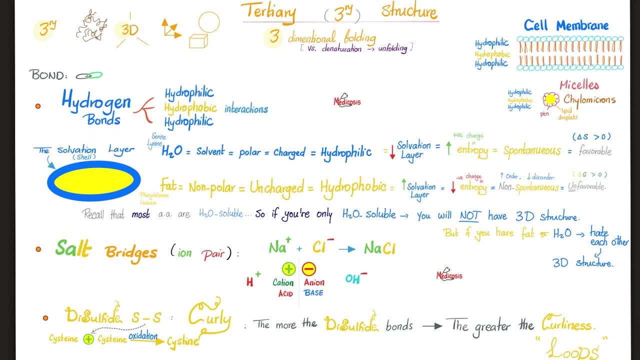 hydrogen bond. Remember the cell membrane. Put the water soluble on the outside and on the inside and bury the hydrophobic, the fat in the middle. Just like this Fat is in the middle surrounded by water, Hydrophobic in the middle surrounded by hydrophilic, This water is forming a shell. 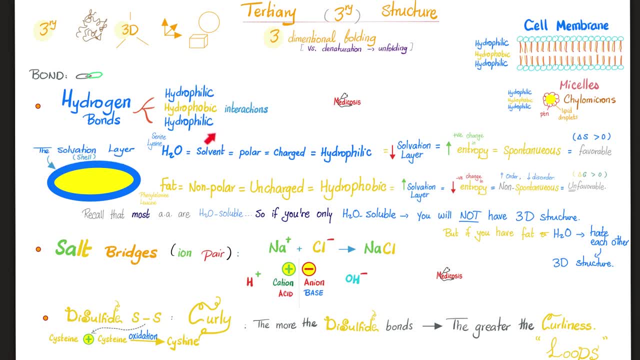 known as the solvation layer. Why? Because water is a solvent. Oh, so the solvation layer is water. Yes, Suppose that this was just water soluble stuff. Do you think we'll have lipid or fat in the middle? No, Do you think we'll? 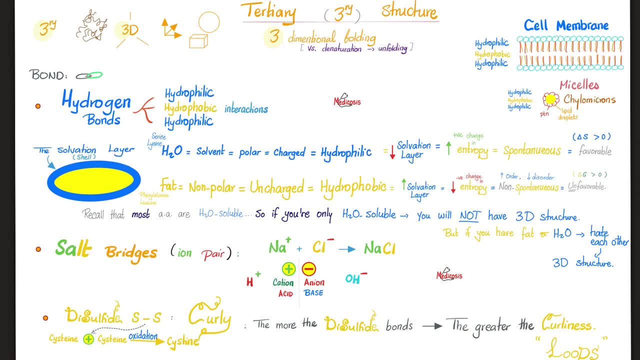 have a shell around it. No, there is nothing to surround. There is no fat to be around, Thank you. Therefore, this beautimous shape depends on the availability of the fat in the middle. Oh yeah, that makes sense. That's why we call them hydrophobic interactions. It's the presence. 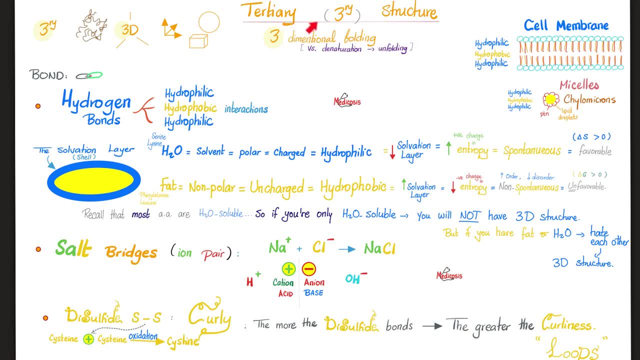 of these hydrophobic residues that give the protein its beautimous 3D structure. Let's review some general chemistry. Water is the solvent and if you are water soluble, you are polar, You are charged, You're hydrophilic. Conversely, if you're fat, you're nonpolar, Uncharged. 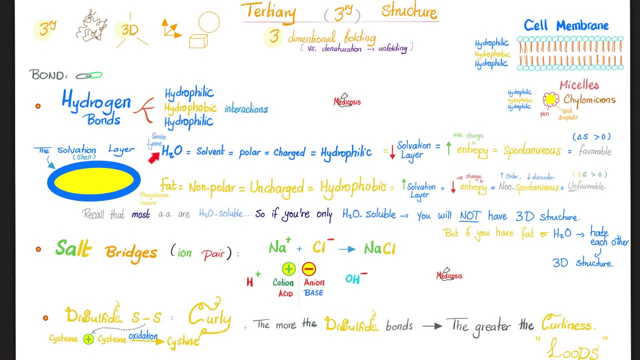 hydrophobic. Let's dig deeper. The more water soluble stuff you have, the less the solvation layer. Why? Because the solvation layer is basically made as a shell to surround the fat. If you have no fat or less fat, You'll have less shell to surround the fat. Duh, Because there is nothing to surround. Okay, I got. 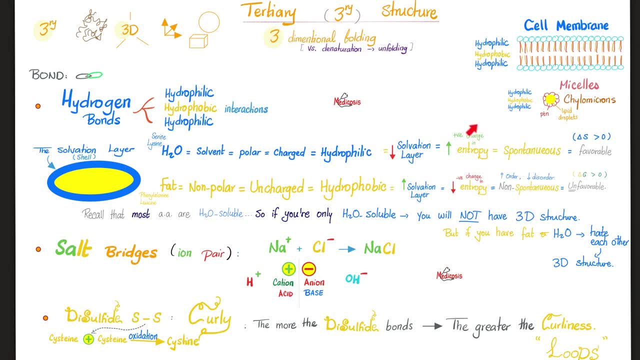 you. And then, when you decrease the solvation layer, you'll increase entropy. We call this a positive change in entropy. What's entropy? Entropy is a lazy butt who's going to hell, For example, when the tea is hot, Okay, that's an active state. And then, as you leave it alone, 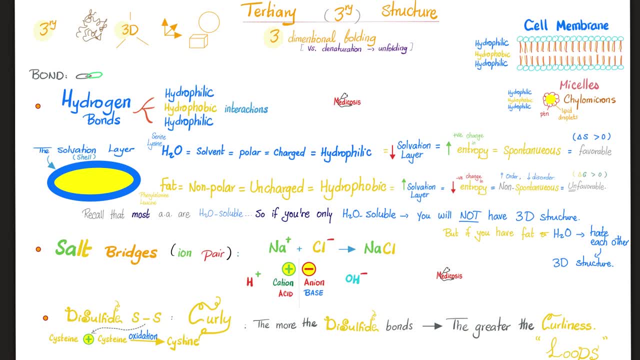 it's gonna go back to the room temperature. Going back is a lazy butt process. It's known as entropy. Conversely, ice melts. As ice melts, it's going towards entropy. So entropy is a spontaneous process and it's favorable because it requires less energy or no energy. Conversely, 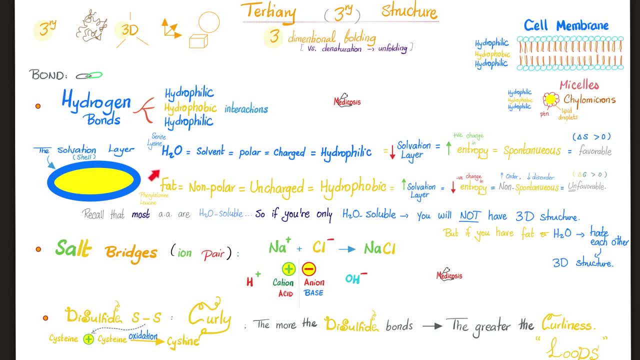 by adding more fat in the middle, you will force the water around it to make a shell. The solvation layer will increase, decreasing entropy, ie a negative change in entropy Because there is less energy in the middle, So entropy. this is non-spontaneous, Unlike the first one And the non-spontaneous 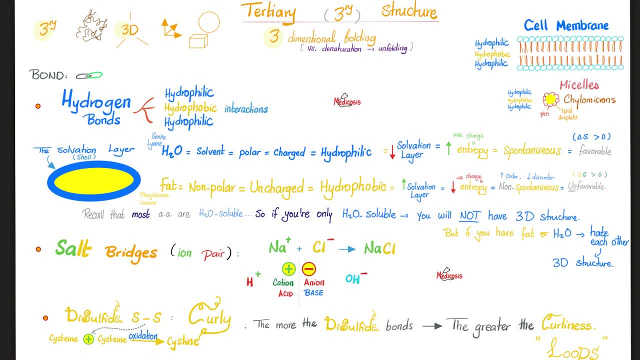 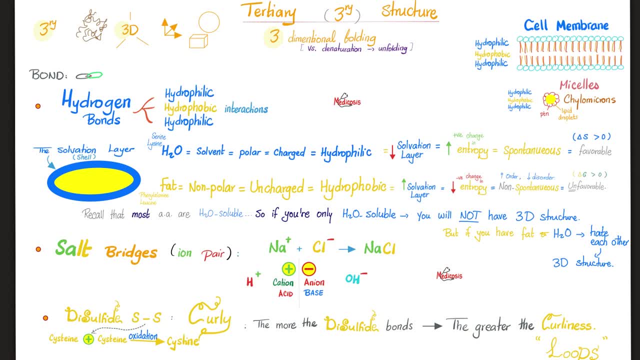 I mean, look at the chalk. I mean look at the chalk. Even acid base have charges. But then when you lump the sodium and the chloride together, Look at this, You get sodium chloride without the charges. Same thing happens to the proteins. Some of those lovely amino acids are positively charged. 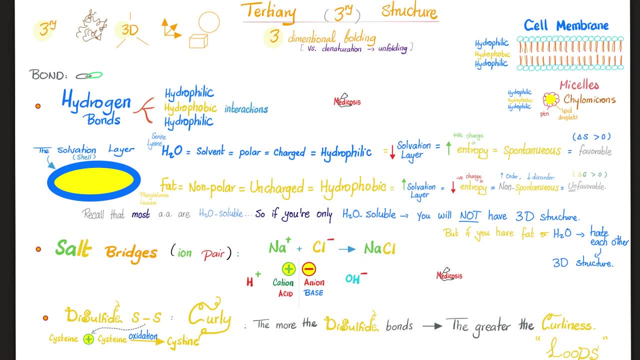 Others are negatively charged And, before you know it, they interact with each other, forming an ion pair, A salt bridge And the crazy mnemonic. again, Yoga bridges are 3d in shape. Why do you wear three 3D yoga bridges to show your curves and curls? Curls, Curly. Why am I curly? Disulfide bonds. 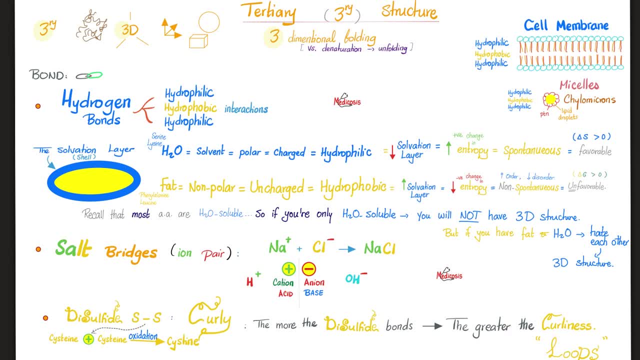 The more disulfide bonds you have, the greater that quote- curliness They make loop in the protein structure. What's a disulfide bond? It's a bond between sulfur and the next sulfur. Example: adding cysteine to cysteine amino acids will give you cysteine. This is a disulfide bond. 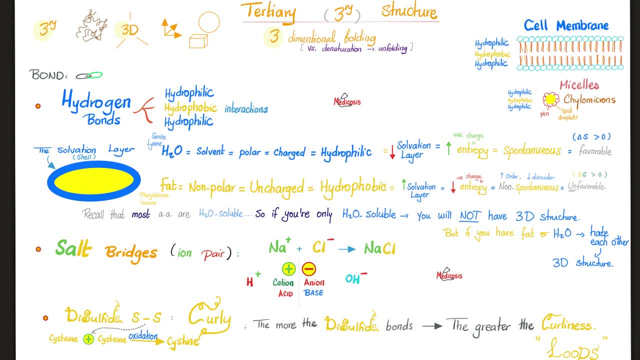 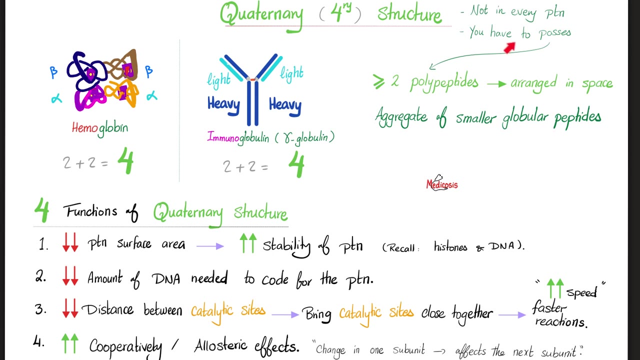 This is an oxidation reaction. Why is it oxidation reaction? Because you lost the electrons. Electrons are negative. When you lose a negative, it's oxidation Lost quaternary structure- Not in every protein. In order to have a quaternary structure, you need to possess. 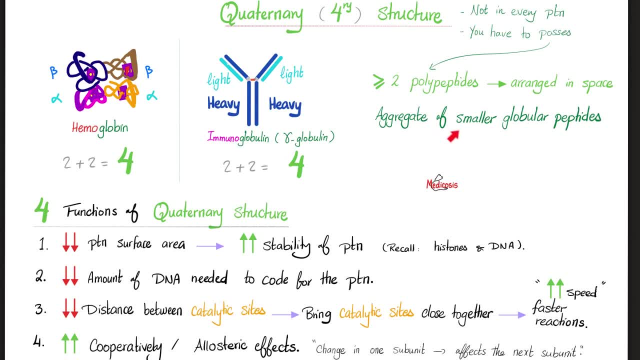 two or more polypeptides. arranged in space, They aggregate to form these lovely shapes such as the hemoglobin with two alpha chains and two beta chains, or the immunoglobulin with two alpha chains and two beta chains, The hemoglobin with two alpha chains and two beta. 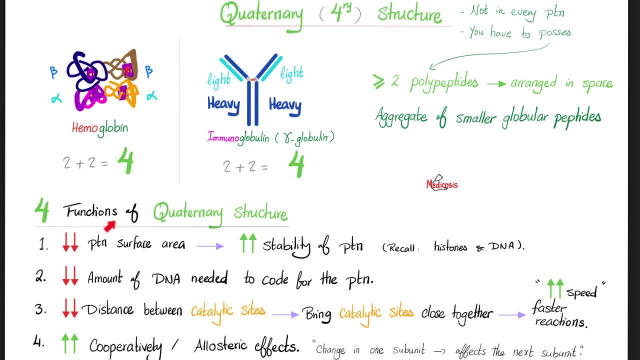 chains. Why do we need quaternary structure? Because they serve four functions. Just remember that I have three arrows going down and three arrows going up. Let's go Look at this. Oh, folding and wrapping and entangling it on top of each other will decrease the surface area. 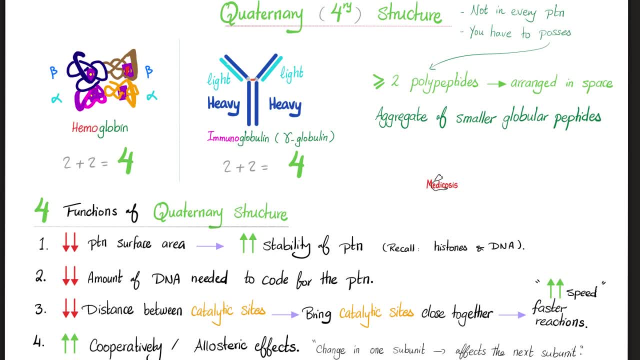 Of course. Conversely, if I unwrap it, if I make it linear, I will raise the surface area, But when I wrap it like this, it's going to lower the surface area, which makes it more stable, by the way, because now not every doofus can come and break it apart. This is a wonderfully integrated structure. Next, it decreased the amount of DNA needed to code for the protein. Well, no kidding, because it decreased the protein surface area. Duh, When I wrap it like this: now, this part came closer to this part. Oh, that's going to be easier for us because you decrease the distance. 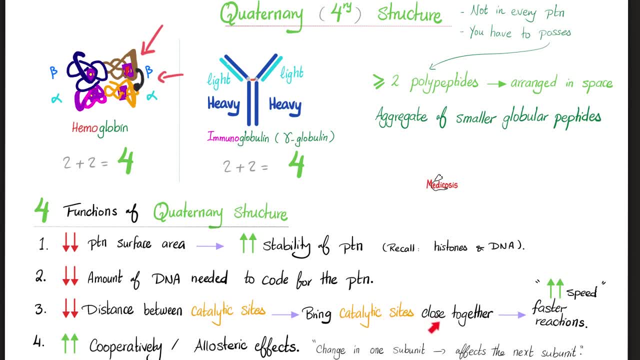 between the catalytic sites. bringing catalytic sites close together giving you a faster reaction With higher speeds lost. they increase cooperativity or allosteric effects. We'll talk about that later, But for now just remember it means change in one subunit will cause a change in the next. 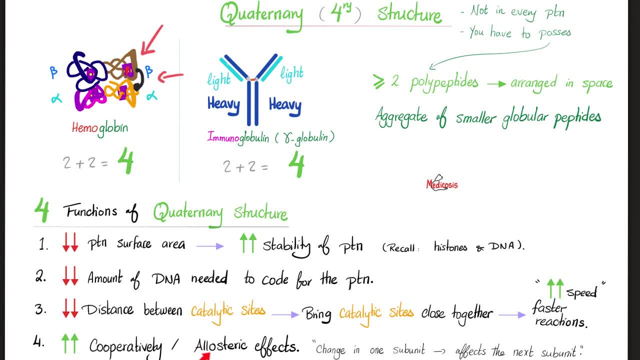 subunit. It could be an activation- We call this an allosteric activator- or it could be inhibition- allosteric inhibitor. There are many doofus pharmacology students who just read the words allosteric activator and allosteric inhibitor.